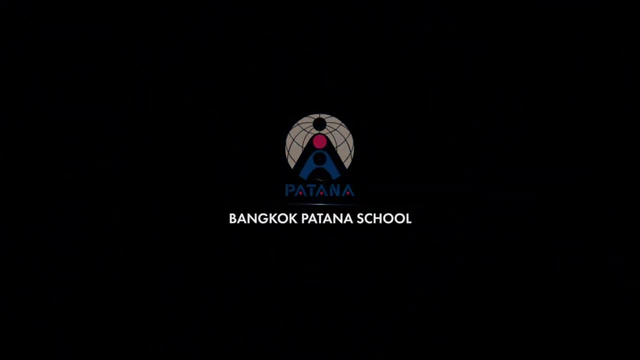 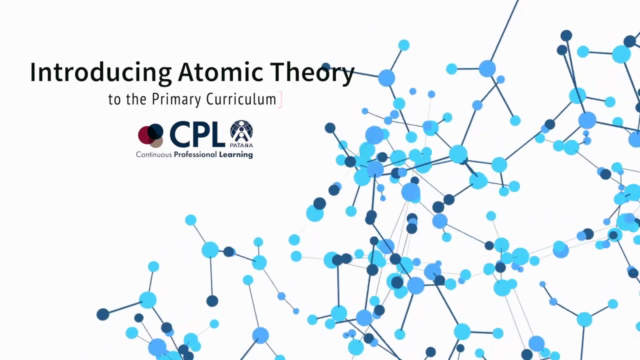 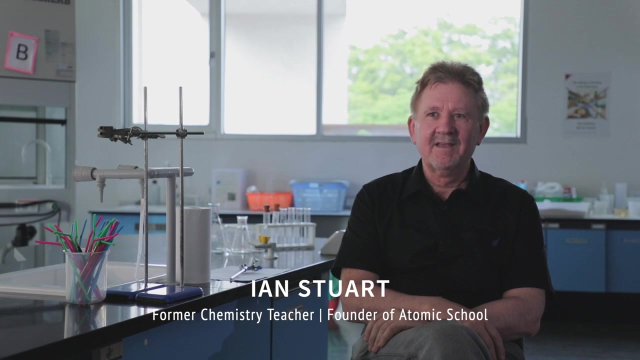 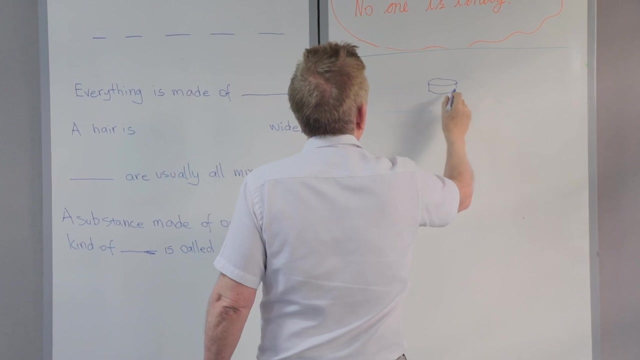 Where did this idea of teaching atomic theory to young children come from? From my son, actually. I was a retired chemistry teacher at the time, and Tom reached the ripe age of about eight years old and he started asking some chemical questions. So I was the 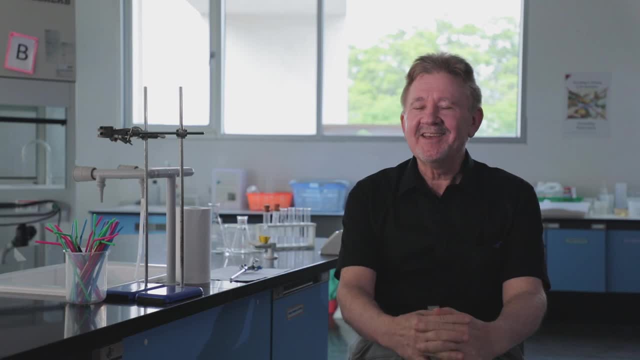 perfect person to give him some chemical answers and he was able to get it straight away. There was a really thorough comprehension of the answers and of the. he had a great ability to understand high school chemistry at age eight, So this kind of surprised me. I went. 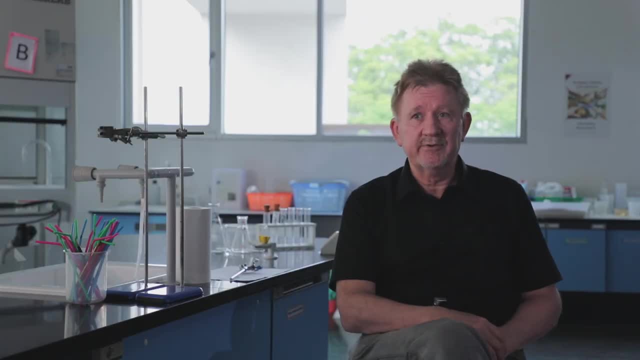 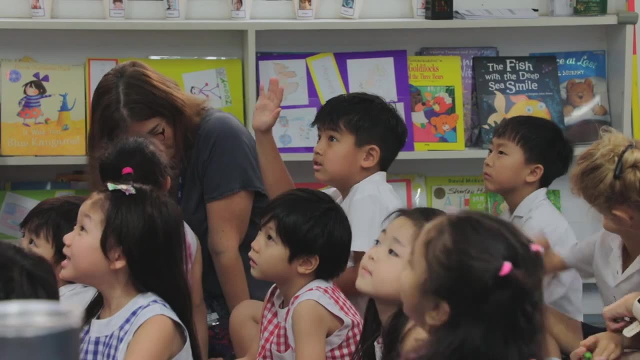 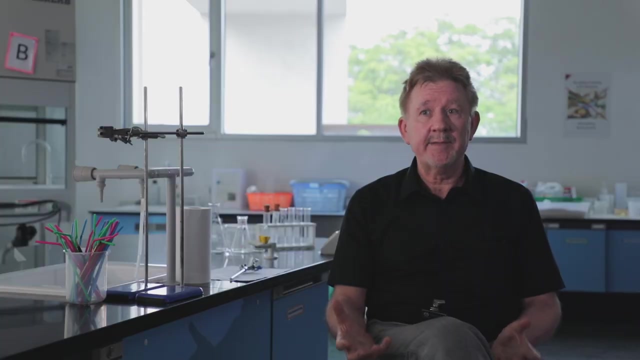 to his school and found that his peers could also understand chemistry at a high school level. So I thought this is a bit weird, really, and surprising, because it means that we're underestimating primary school students. They can, they are capable of much higher levels. 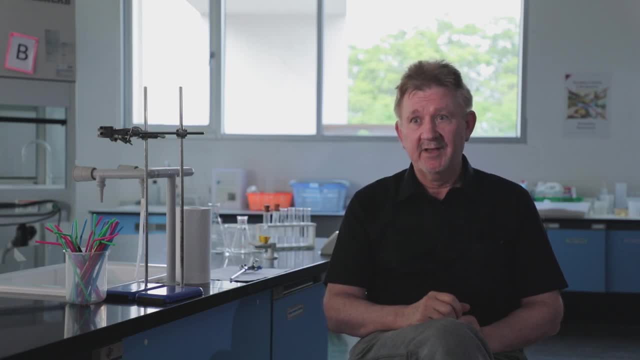 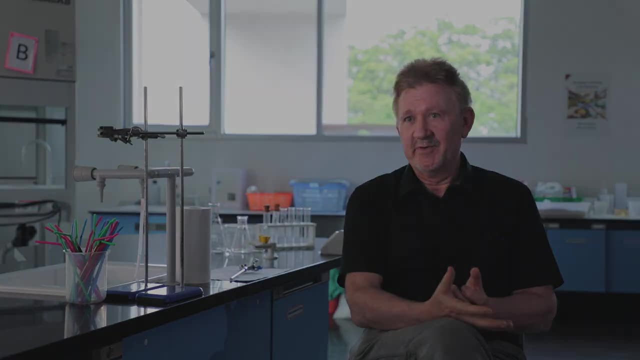 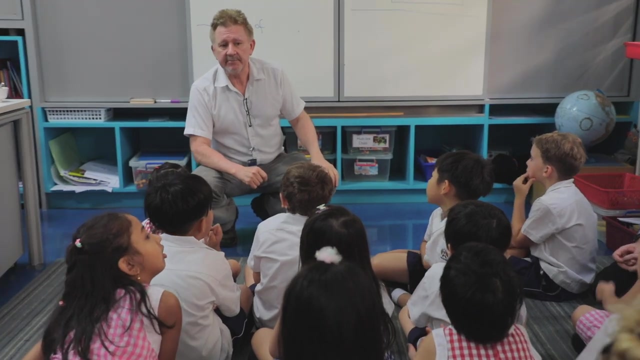 of understanding than we are giving them credit for. It's developed from there. I went into his school, started teaching high school chemistry- there atomic theory- and then I went to his school as well. You're actually right: Everything in the world is made out of atoms And we 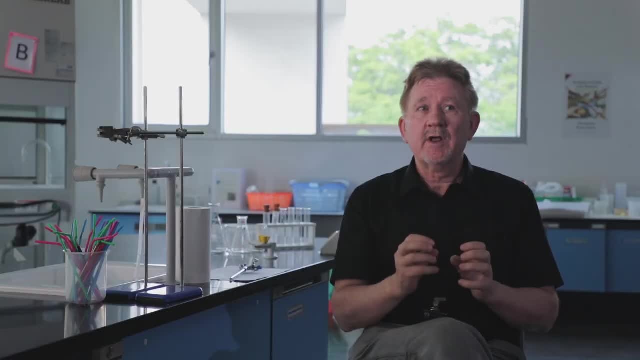 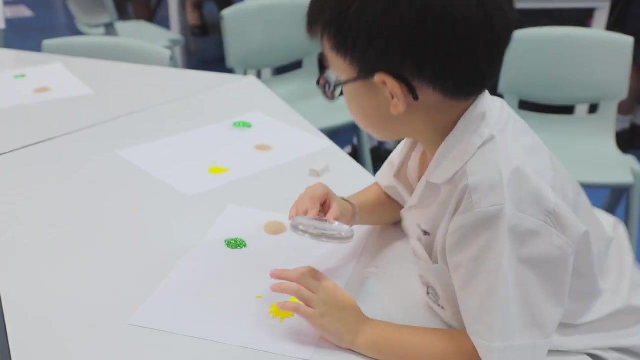 developed resources that were adapted to primary school kids and also primary school classrooms, because they don't have wonderful laboratories like this. So we needed experiments that could be done in very simple conditions. Also, we needed materials that were able to do a lot primary school teachers could engage with, because they have proven themselves to be. 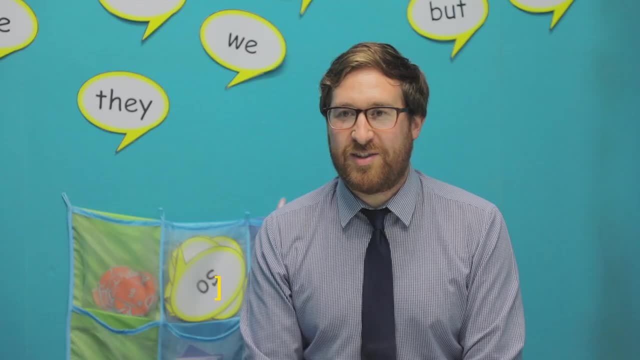 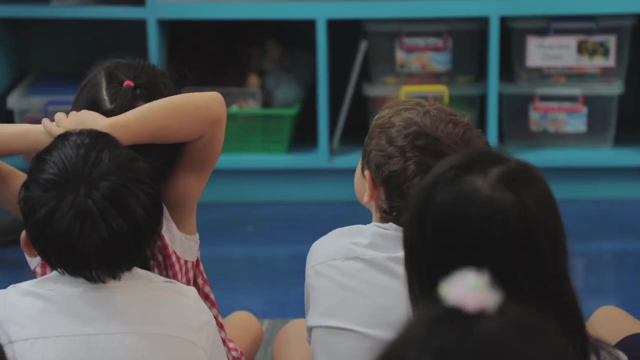 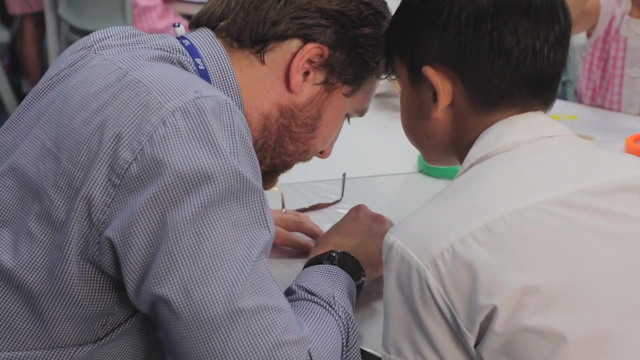 wonderful at teaching atomic theory. I can say definitely the children are ready. I was worried that the abstract ideas might kind of go over their head a little bit, but the way it's explained in a very simple way, using concrete resources and the microscopes, has really helped them to understand, I think. 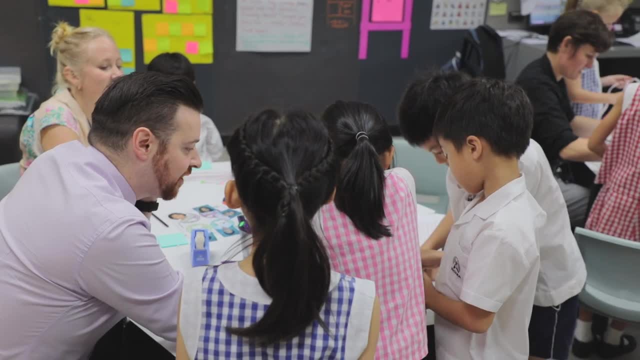 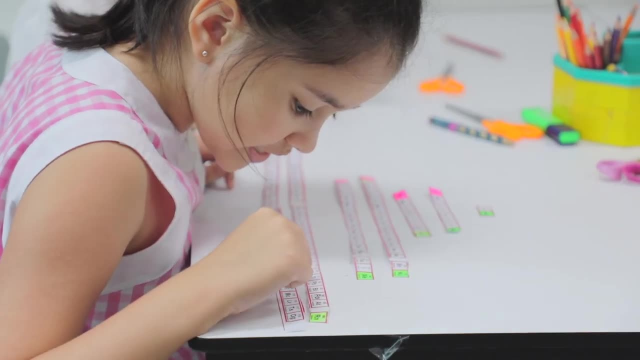 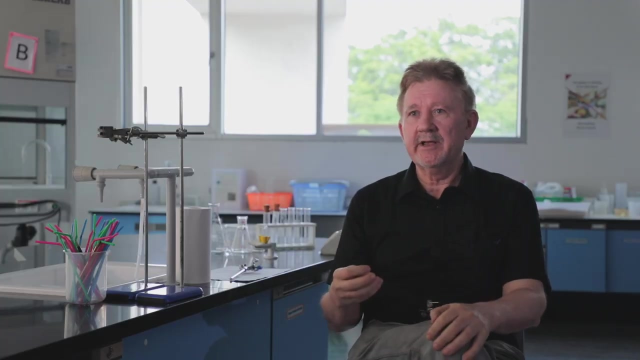 they are ready. Because I'm a high school teacher, I don't have all of the pedagogical skills for communicating with primary school kids that they have, So it's a wonderful combination for a primary school teacher to upgrade their understanding in this area and teach this brilliant stuff. 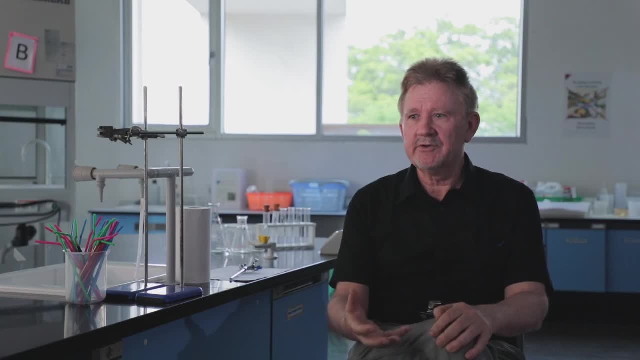 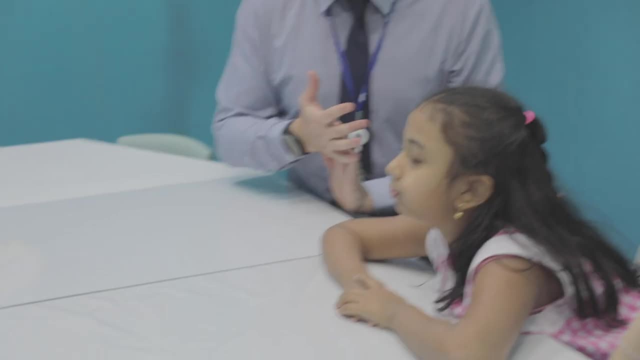 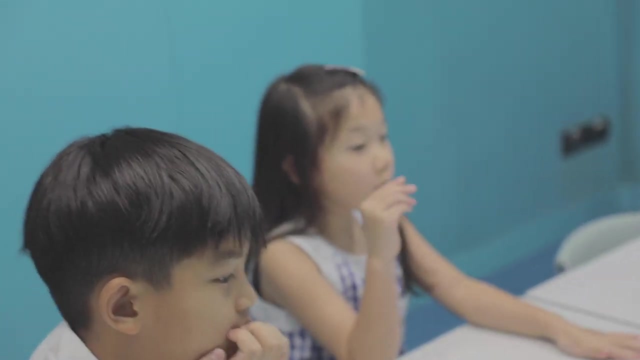 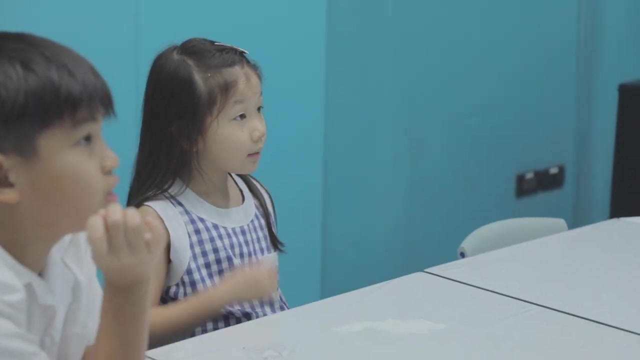 that will enable their students to go on to much greater success in future science education. I have some really really, really super duper little things in the even, in tables and everything. What about in my hair? Yeah, Smaller than an inch. 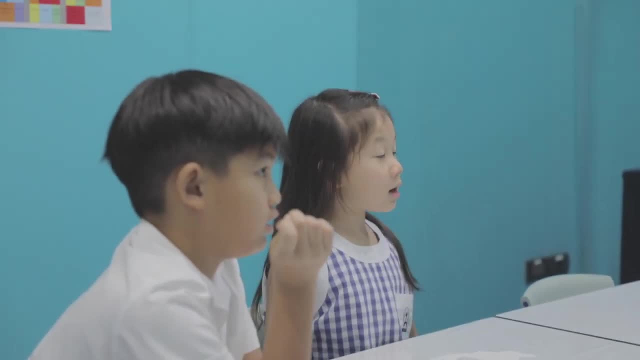 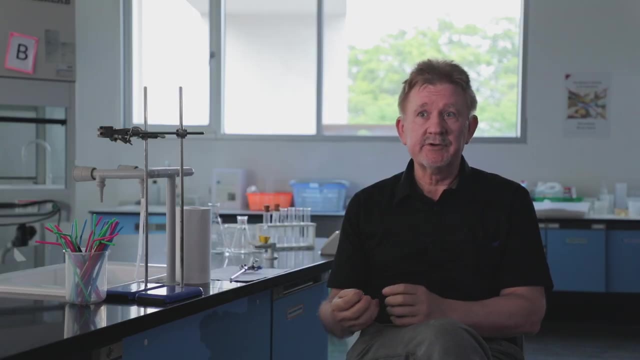 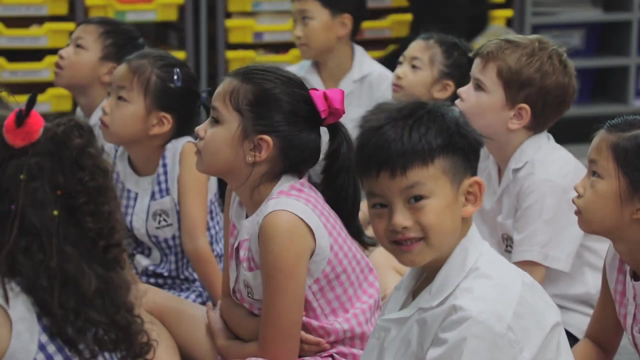 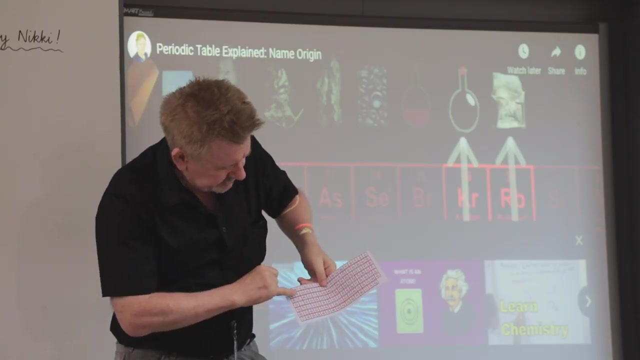 Yeah, What about my glasses? Everything in this room There are, and were, a lot of sceptics, which is why we got the University of Southern Queensland involved. Yeah, We researched the program so that we had empirical evidence that kids understood atomic theory at primary school level. So we established that as a matter of fact rather than as a 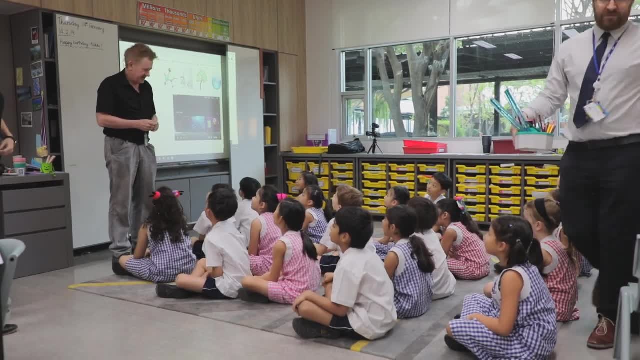 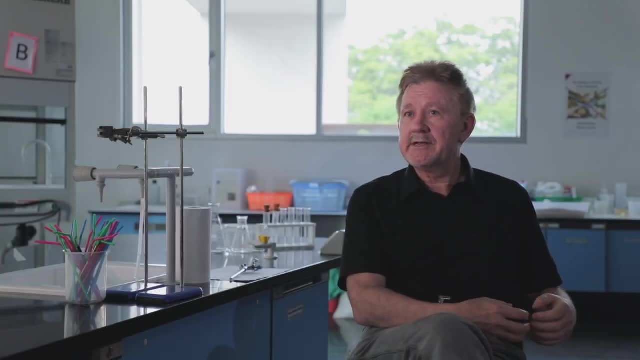 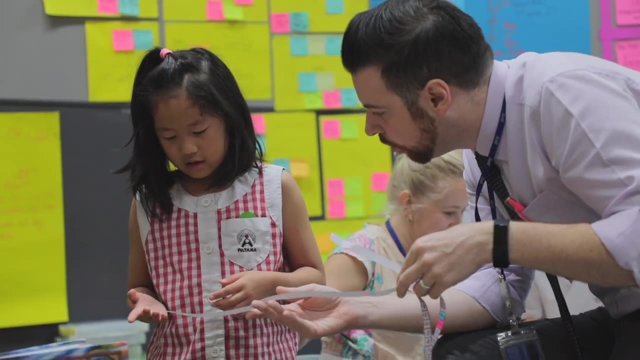 matter of opinion. Are you an element? No, No, How come? Because there's more than one atom. So this provides this is attempting to open the gates, to allow, give permission to teachers and to schools And to parents to let their students understand this and learn about this, which they absolutely. 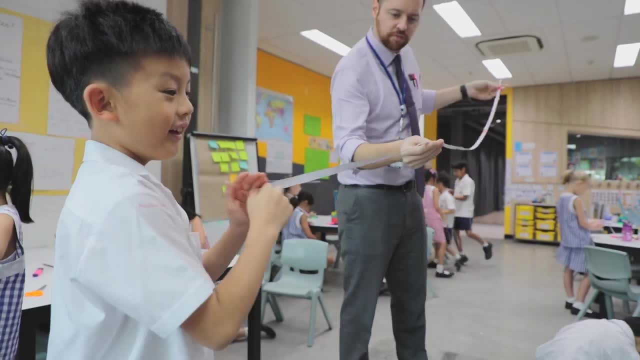 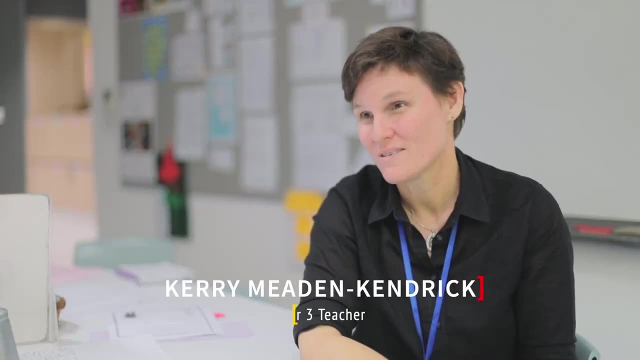 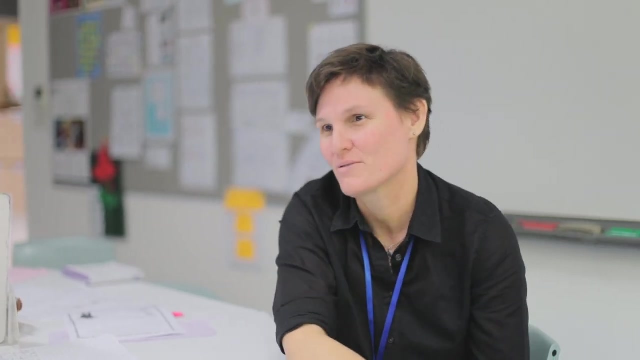 are craving to learn about and understand. The curiosity of students in this area is just amazing. The initial session that we had on Monday was really, really interesting to watch, because Ian started really really slowly and he walked them very, very gently through. 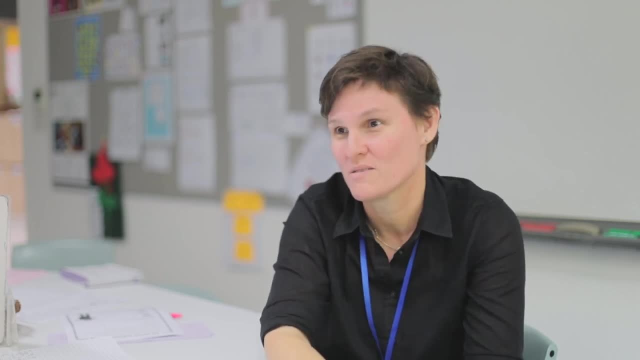 So by the end of the first 10 minutes he got to the point where he was explaining to them. if they really wanted to see one atom in an apple, the apple would need to be the size of the earth, And that blew their minds. 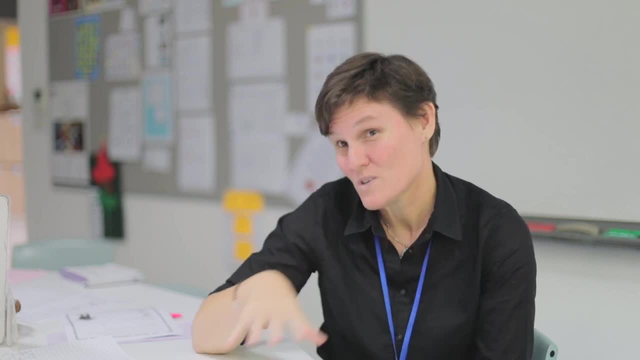 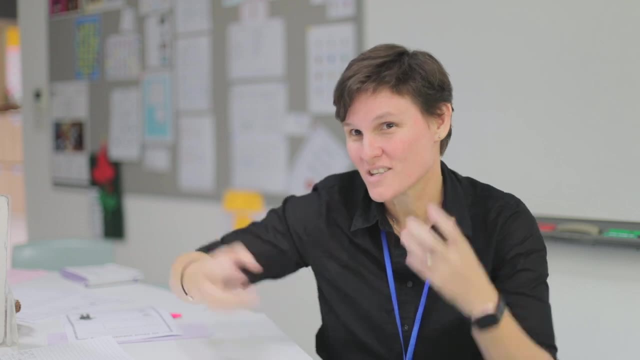 So he had them hooked right from the start. So it was very, very hands on. It was very, very engaging And they learned masses. They were so thirsty for that knowledge as well. So for lots of them it was completely new learning, which is so rare in their learning. 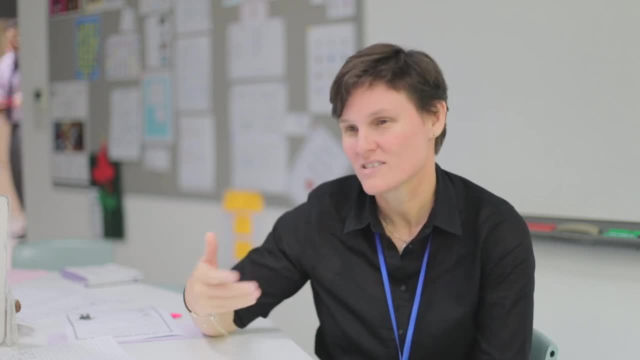 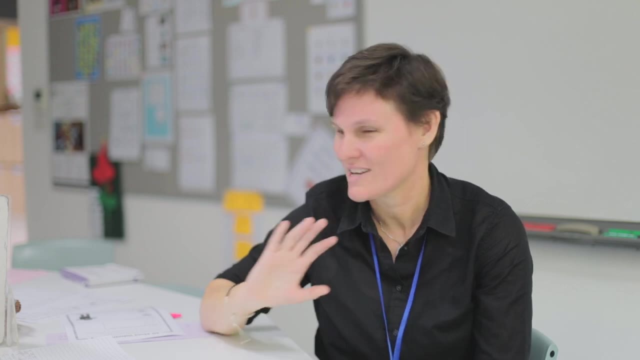 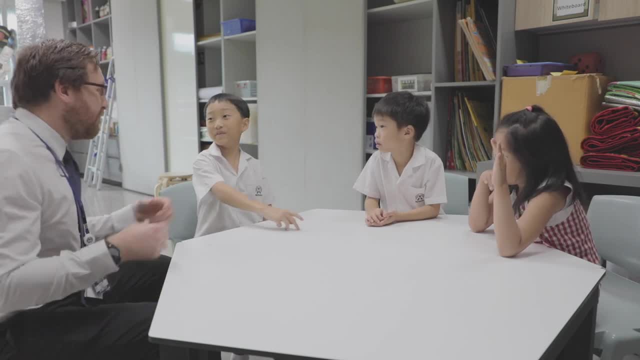 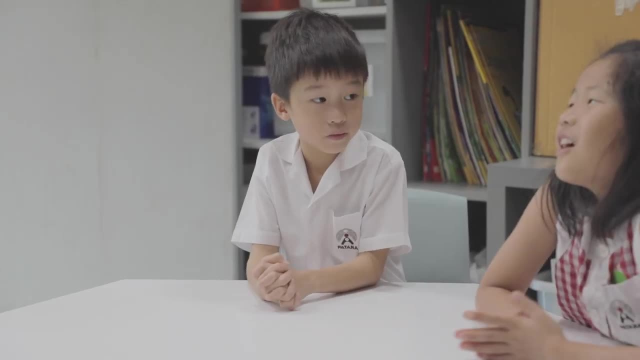 Thank you. Yeah, what did you find a bit tricky In making a table on there? Making the table, there were lots of steps, weren't there? So cutting and coloring different parts. What would you change about today's lesson? make it even better? 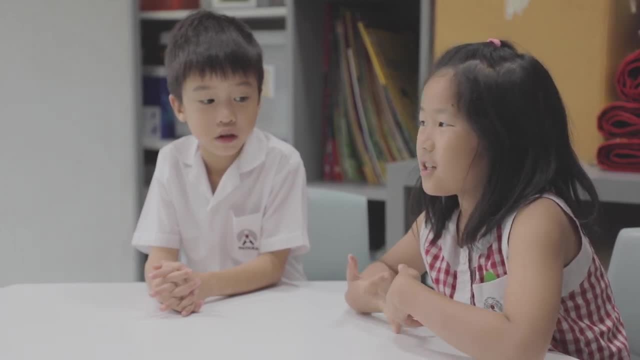 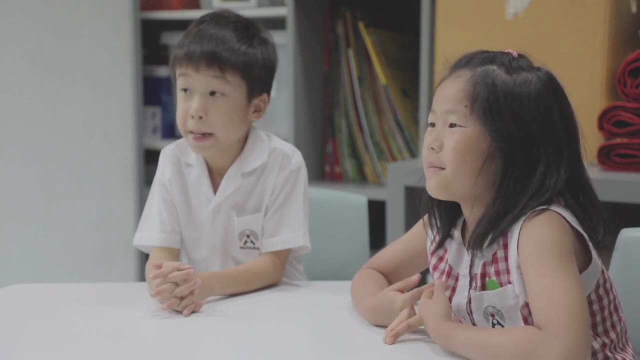 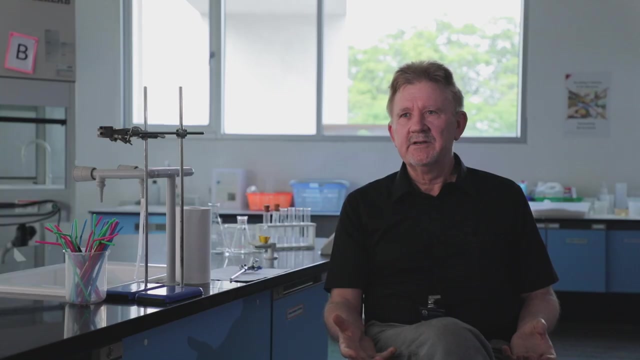 Get all of the 118 elements and actually find the atoms in them. So to actually see the atoms. do you remember the name of the microscope that we would need, Electron microscope, мозes Electron microscope. So we've been withholding it from them until high school. 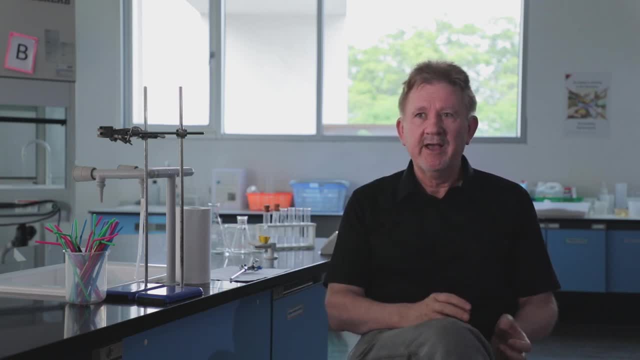 and there's no need. We've got this opportunity to go in and allow students to explore this wonderful area of science. In fact, it's not just wonderful, it's the foundation of science. It's interesting what we introduced them to this concept. 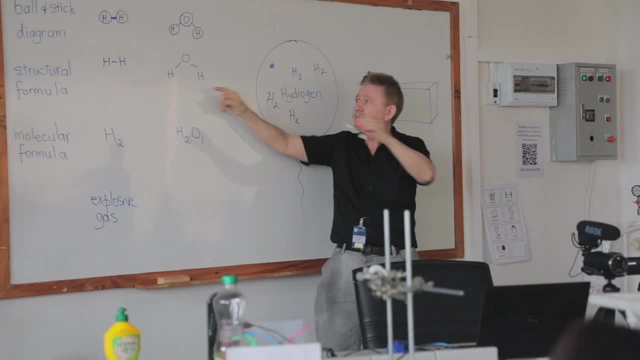 in the sense that it's something they want to know. You talk to them about, oh, we're gonna do molecular science, and they're like: oh, what do you mean by that? Let's do? oh, it's gonna be the periodic table. 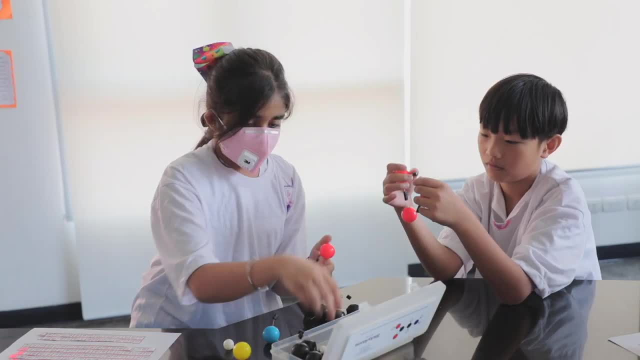 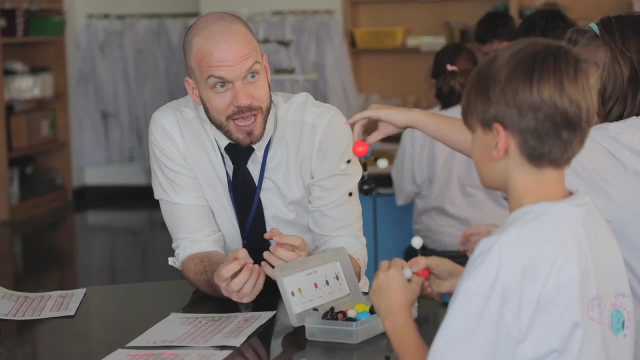 And you're like, oh okay, and their interest sparks. Then you start talking to them about these different elements and you talk to them about weight And they're getting all this knowledge. Now I envisage that it moves on to this: 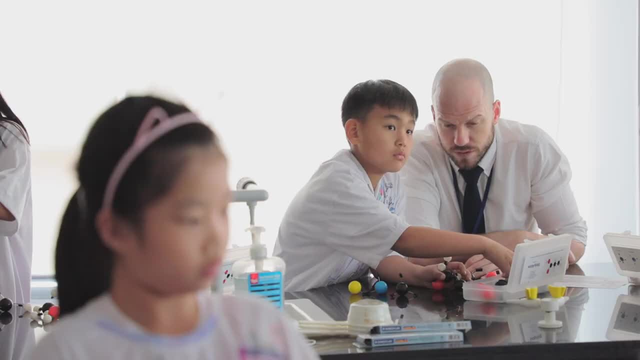 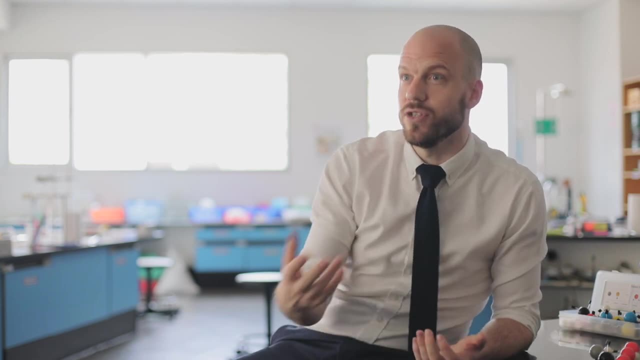 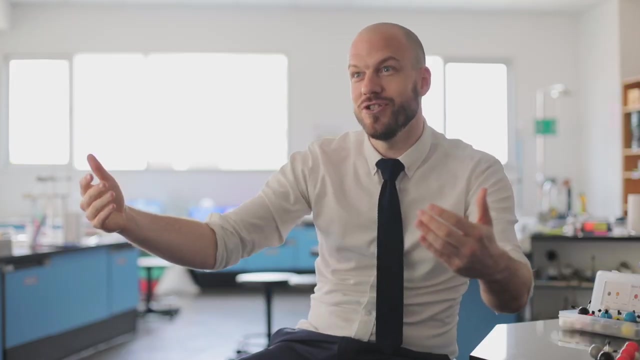 within the curriculum in the sense that we link it back to some sort of skill of investigation. So when we move into things like reversible and irreversible changes, where chemical reactions are coming involved, they'll be able to see that, for example, when they're combining wood and oxygen. 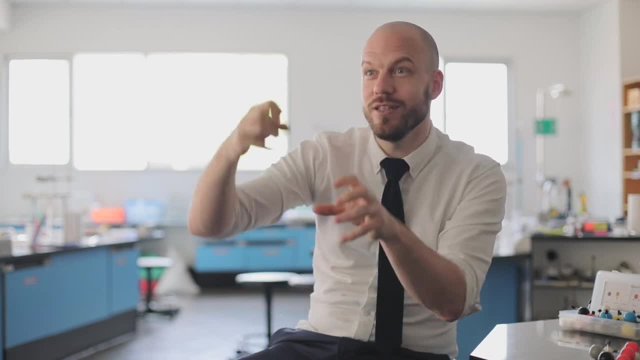 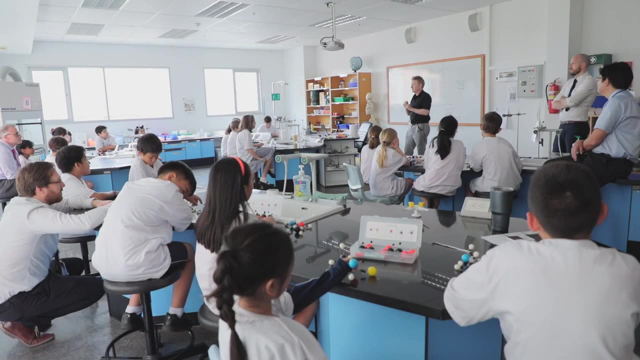 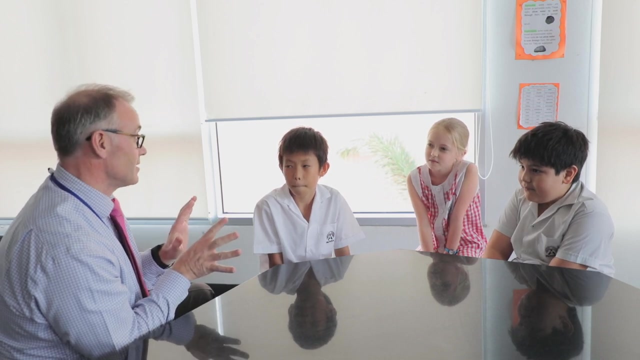 to make fire. fire isn't actually an atom, but actually then they get some byproducts from that chemical reaction that are irreversible And fingers crossed. it would then help them to understand the science behind the reactions that they are looking at, If you could change anything about the lesson. 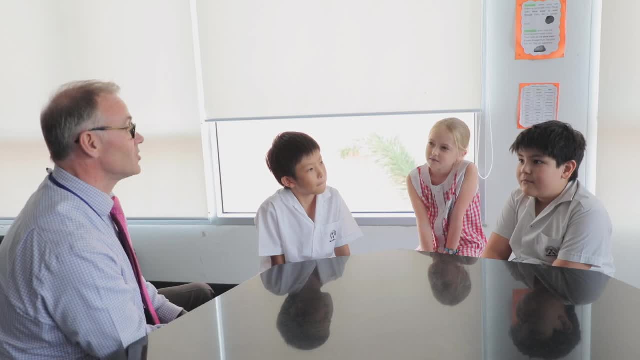 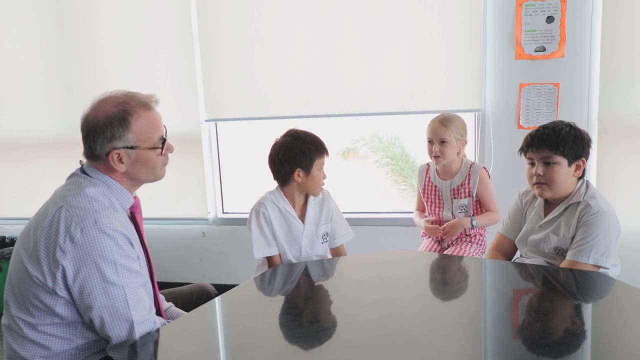 to make it even better. what would you like to change? Try to communicate more, because it was hard to talk with my partner at the same time as putting it together, because, well, if she already did it, then it gets like really confusing.